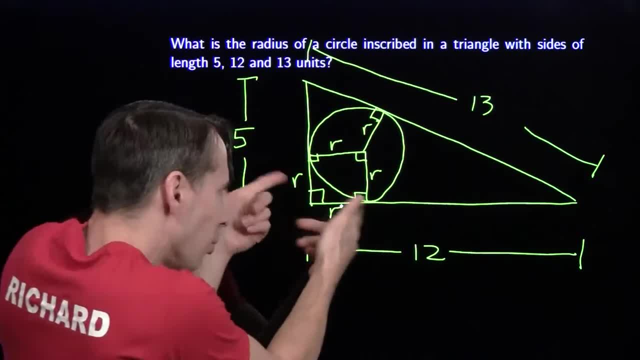 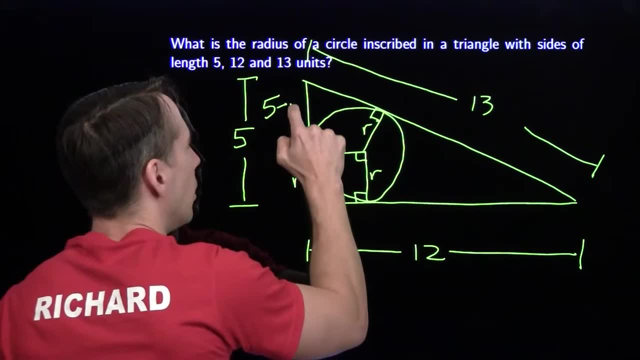 And once I figure out something new, I think, hey, do I know anything I can use with that? Well, I see this r that I just discovered. I know that this whole thing is 5, so this up here is 5 minus r. Use that same strategy over here. It tells me that this length right. 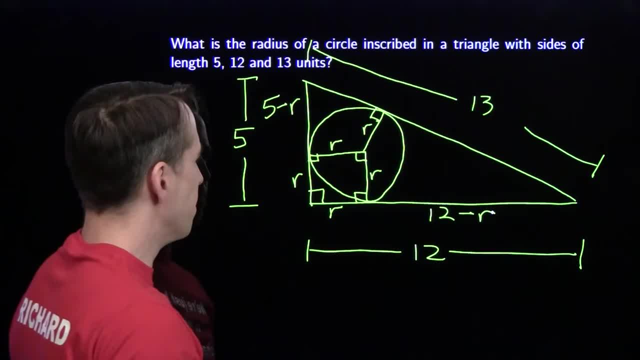 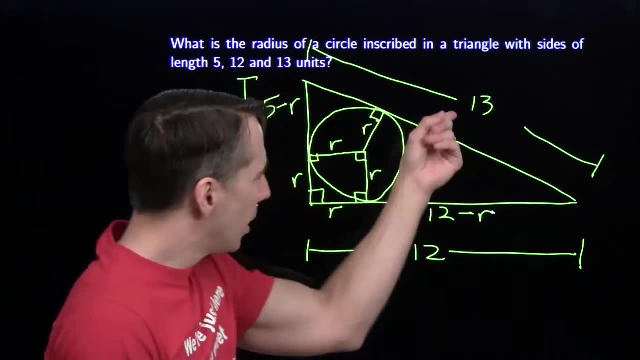 there is 12 minus r. Hmm, Seems a little stuck. Another key strategy here is, I think: what piece of information have I not used yet? I haven't really used this 13. that's sitting over there, So I'm going to look along here. 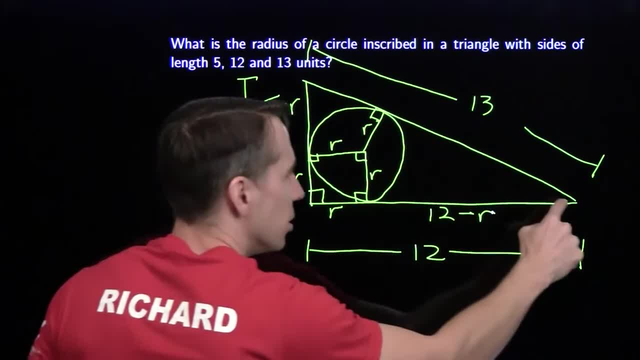 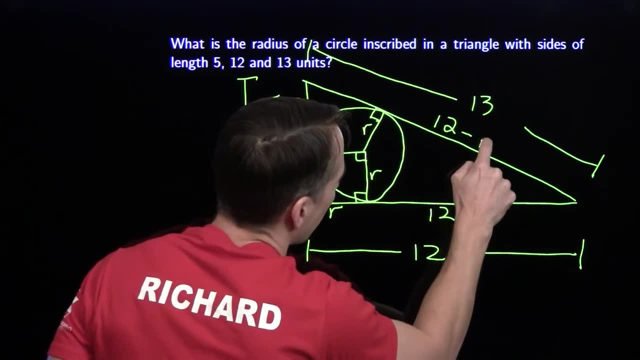 I'm going to see. this tangent is equal in length to this tangent right here, So I know that this length is 12 minus r. Use that same strategy again up here. You know, whenever I use this strategy and I learn something, I look for another way to use that strategy. 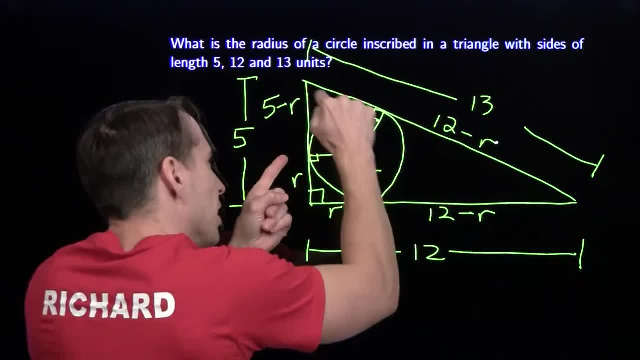 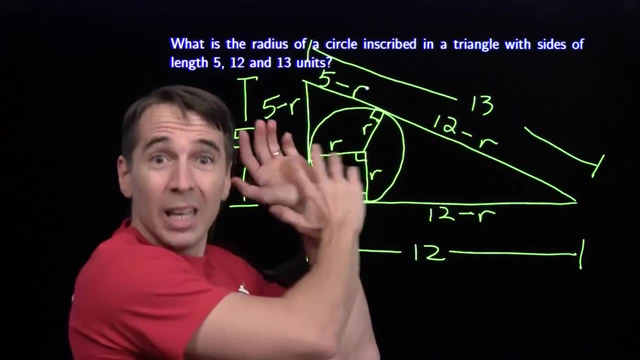 right away, It might have more to give. Take this: 5 minus r equals this segment. over here It's also going to be 5 minus r. Now, one of the reasons we draw a diagram label: everything is what we're hoping to. 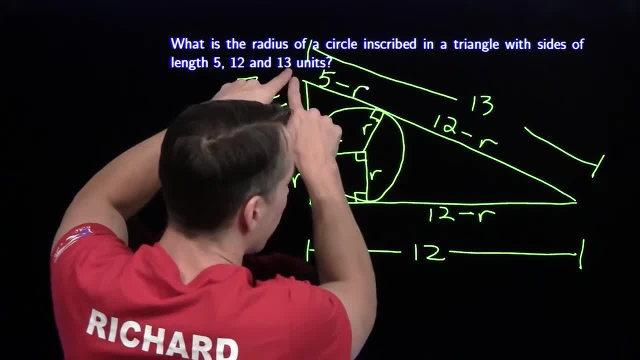 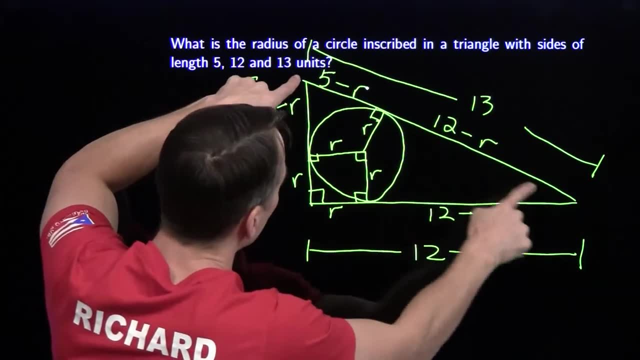 find is two different expressions for the same thing. I've got two different expressions for this length right here. First it's 13.. And then, second, it's the sum of these two, 5 minus r plus 12 minus r. So I can add these two together: 5 minus r plus 12 minus r gives 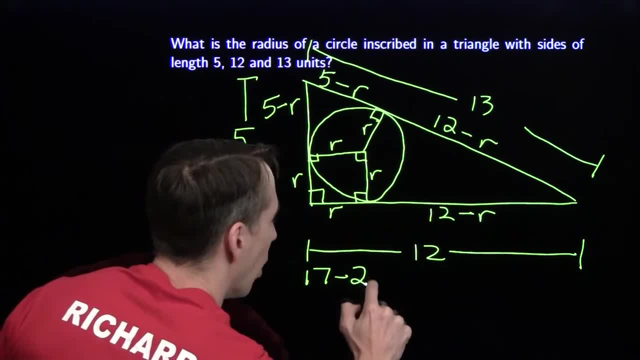 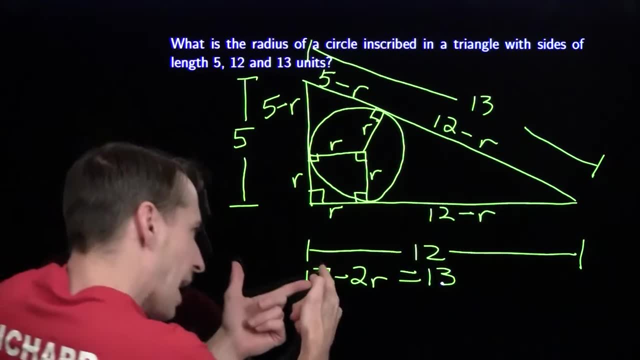 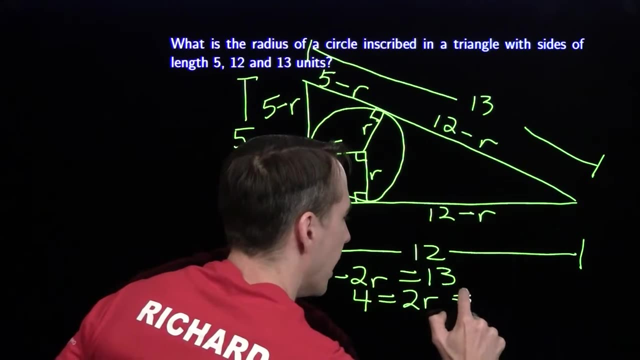 me 17 minus 2r, Just adding these two together, And that has to equal 13.. So now I just add 2r to both sides, Subtract 13 from both sides and I have 13.. I have 4 equals 2r, And that tells me that r is 2.. And since I used my variable for the 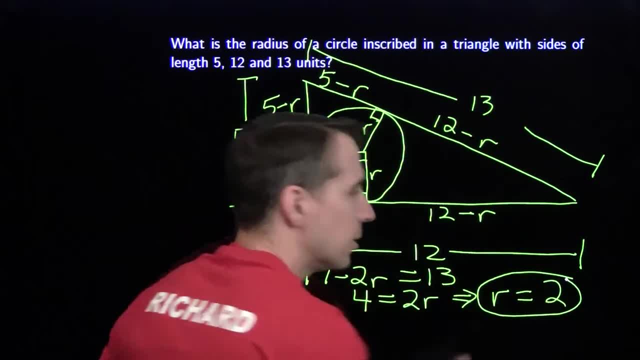 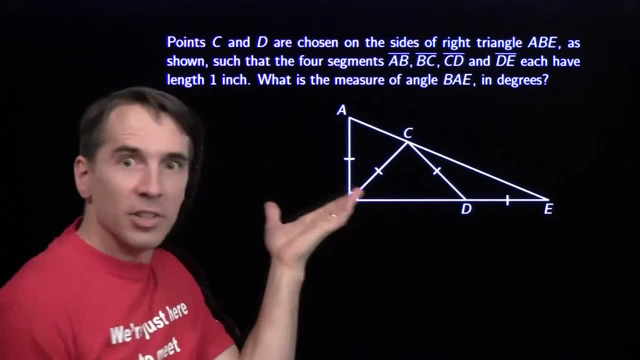 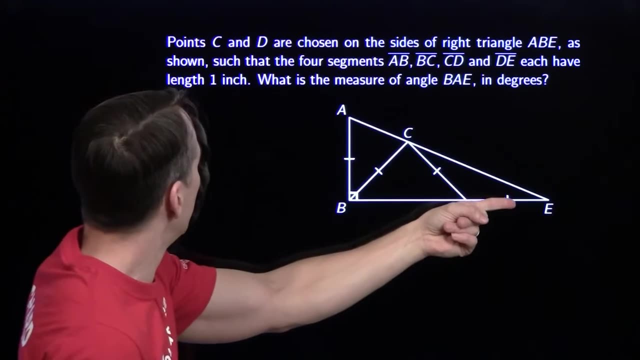 thing I'm looking for. I can just write down that 2 as my answer. I'm ready for the next problem, All right. well, here they gave us the diagram. That's awfully convenient. The points C and D on the sides of a right triangle have another right triangle here, ABE, such that these 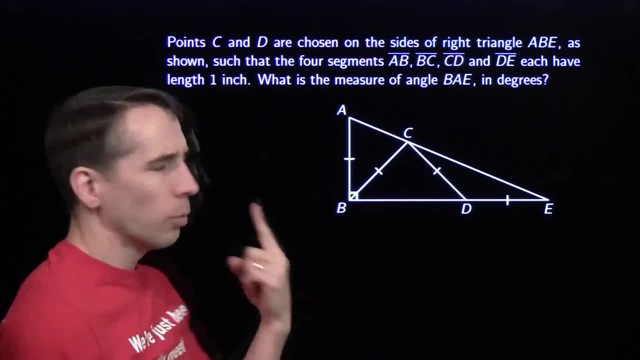 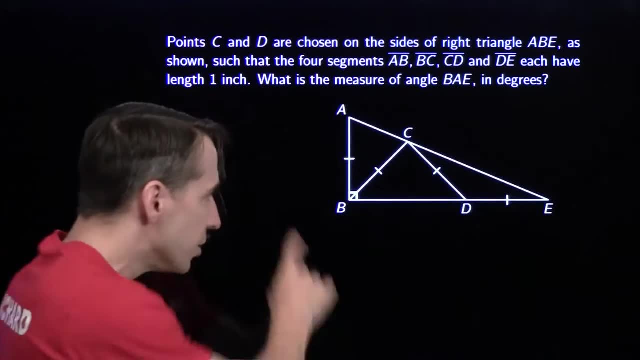 four segments Each have length 1 inch, So they're all the same length. I got them all conveniently marked in the diagram for us. If they hadn't done that, that should have been. the first thing you do is mark everything, so you know what's equal, And we're looking for the measure of 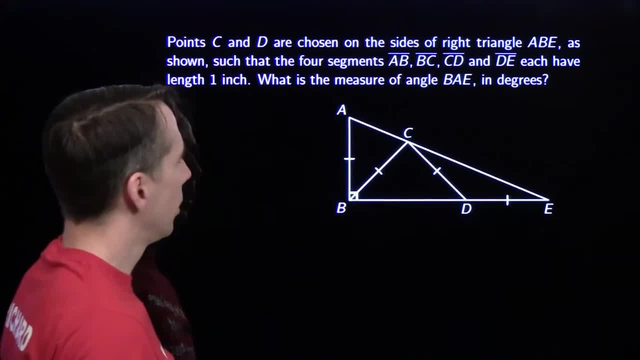 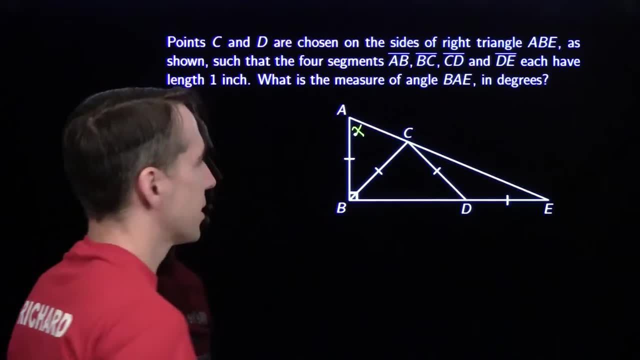 this angle, BAE, And once again we're going to assign a variable to the thing we're looking for. We're looking for this angle right here. We're going to call that x. Now let's go looking for other things. we can find. We have an isosceles triangle right here that tells me that this is x, And 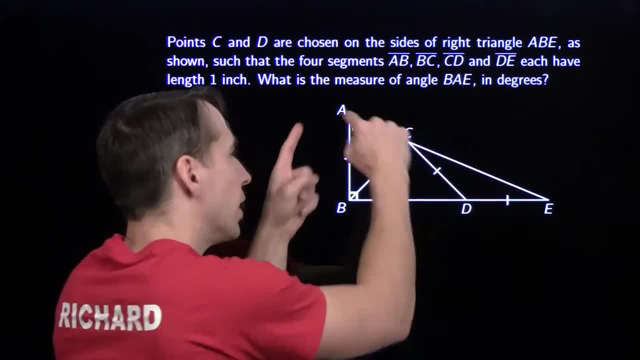 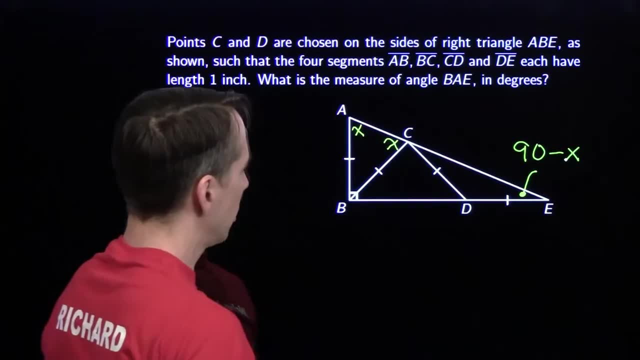 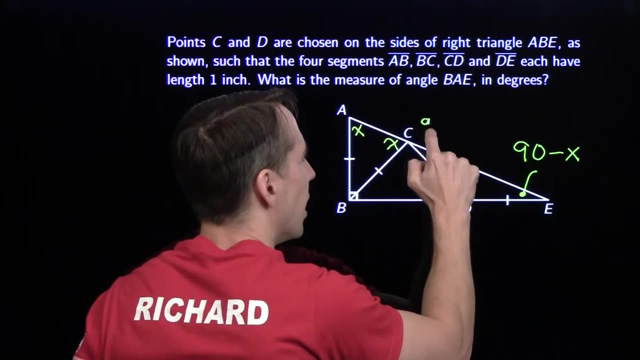 we're going to call that x And we have the right triangle right here. that tells me that this angle over here is 90 minus x. And I have another isosceles triangle right over here, so that tells me that that angle is also 90 minus x. 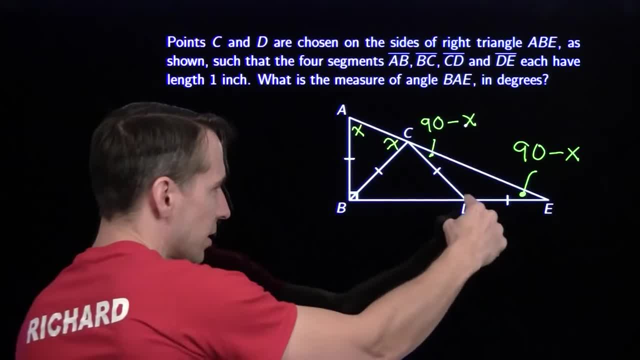 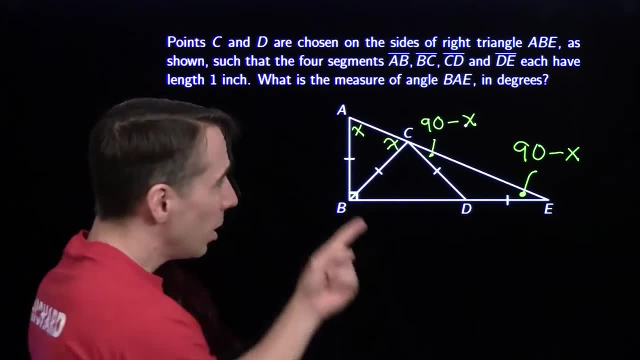 Now, there are a whole bunch of things I can figure out. I can figure out that angle in terms of x, that angle in terms of x. I can also go after this one. I'm going to choose this one up here because I see that these three angles have to add to 180, but these 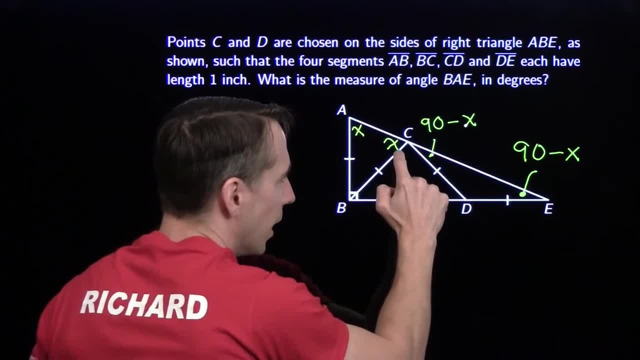 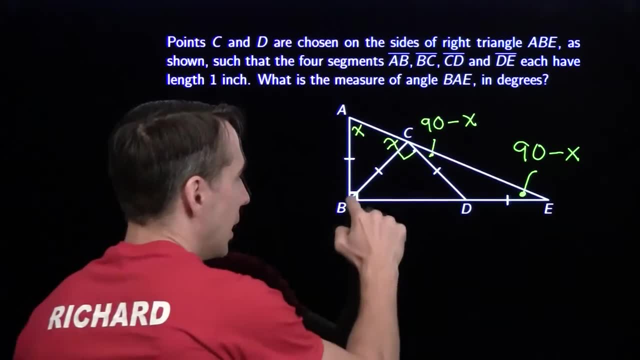 two angles add to 90.. That tells me that this is a right angle, so that when I add these three together I get 180.. That's a right angle. We like right angles. This is an isosceles triangle. isosceles right triangle. That tells me that these two are. 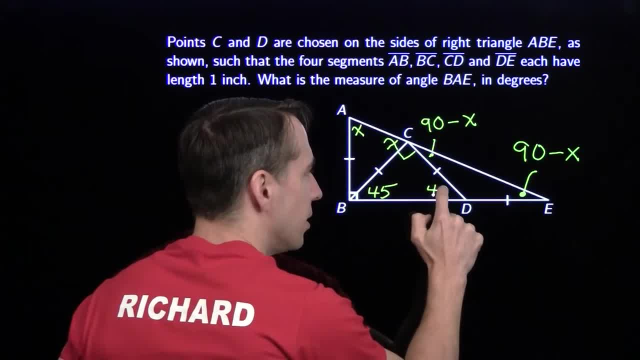 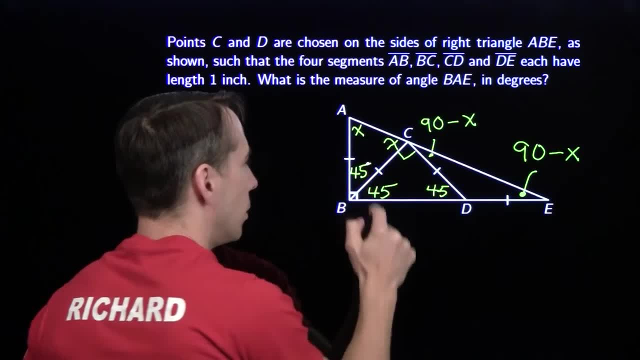 45.. Again, all I'm doing is just writing down the things as I discover them, Since these two are 45,. well, I know what this angle is. This angle is 45, because these two have to add together to 90, and this one is 135, because these two have to add together. 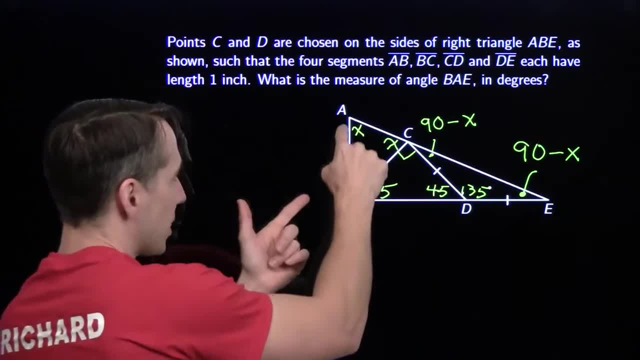 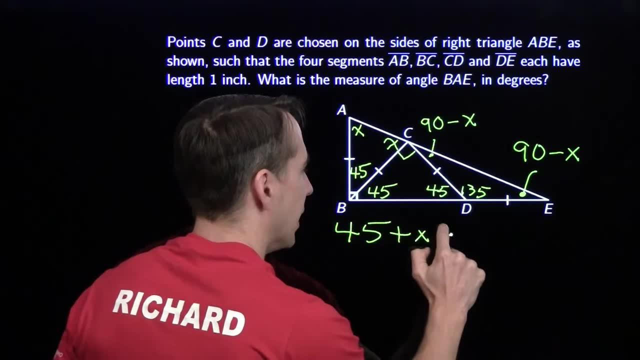 to be 180.. Now I've got a bunch of ways I can figure out x. I'm going to use this triangle right here. We add up these three angles have to get 180.. Again, all I did here. key strategy is to start labeling things and hope for something. 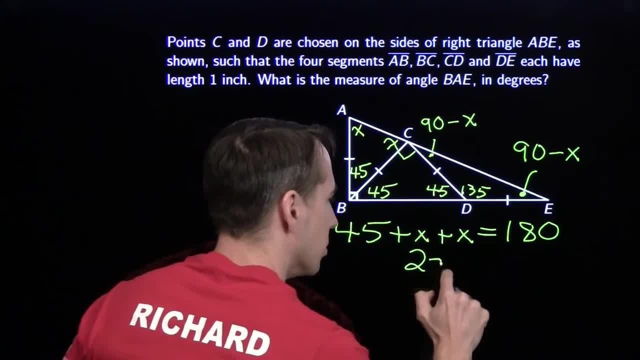 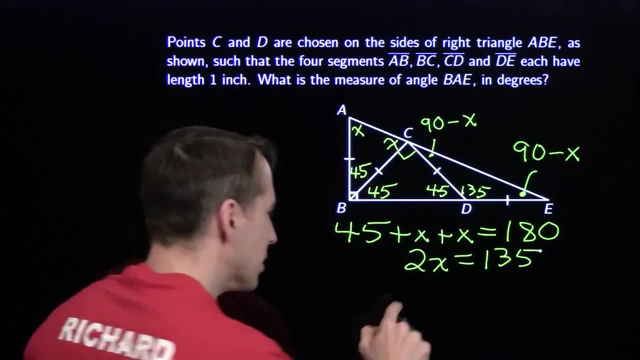 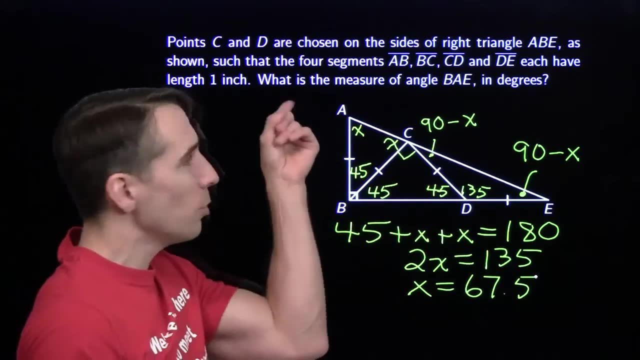 good to happen Over here. I can combine these two x's and get 2x. Subtract 45 from both sides, I get 135.. Divide both sides by 2, and we get our answer. x is 67.5, and since we used the variable as the thing we actually wanted to find, we